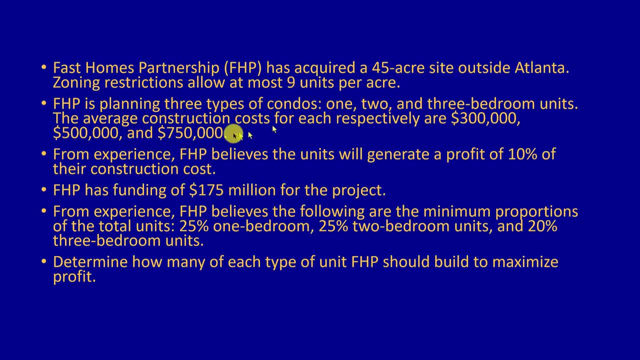 can build no more than nine units per acre. They want to build condos there, one, two and three bedroom units- and they've estimated the construction costs will be $300,000,, $500,000, and $750,000, respectively. for those From their experience, they think 10%. 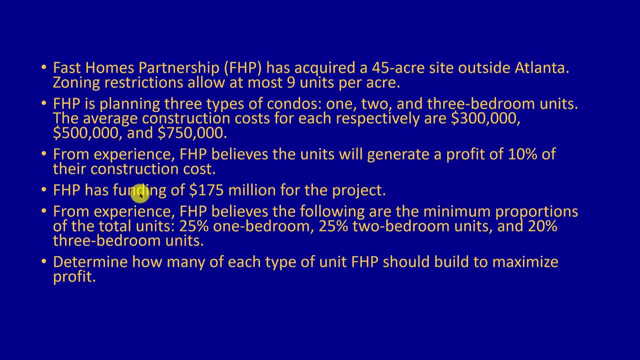 of the construction cost will be the profit. They have funding of $175 million and, from their experience, they think that the best mix would be a minimum of 25% of the units to be one bedroom, 25% of the total number of units to be two and the 20% minimum to be. 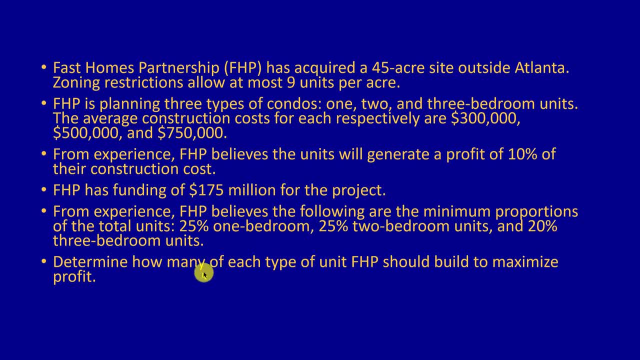 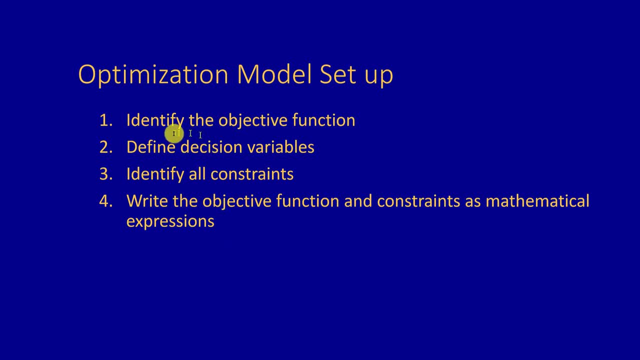 three bedroom. So we need to determine how many of each type to maximize The basic procedure for an optimization model. we identify an objective function. In this case that's going to be. we want to maximize profit. We need to define the decision variables, the things we can change. We need help. 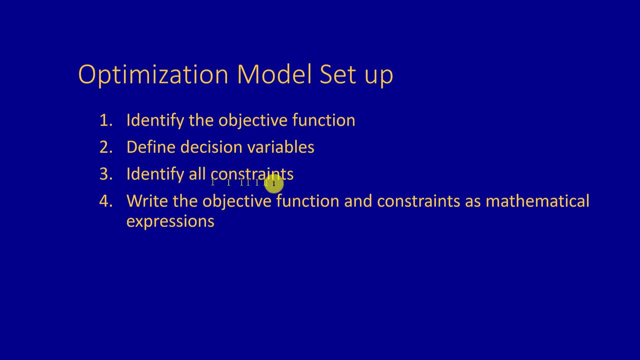 deciding how much to change them. We've got to know all the constraints, and then we've got to write these objective function constraints as mathematical expressions, and we're going to do that in Excel. So let's boogie on over to Excel. 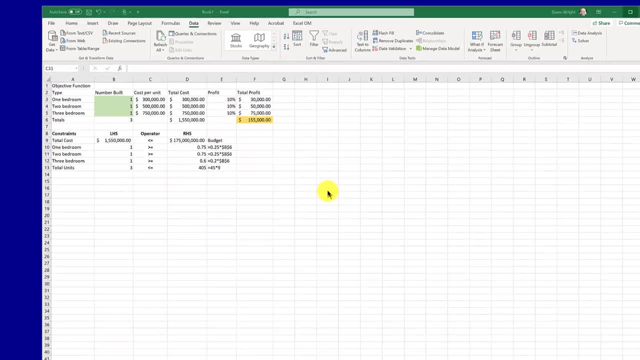 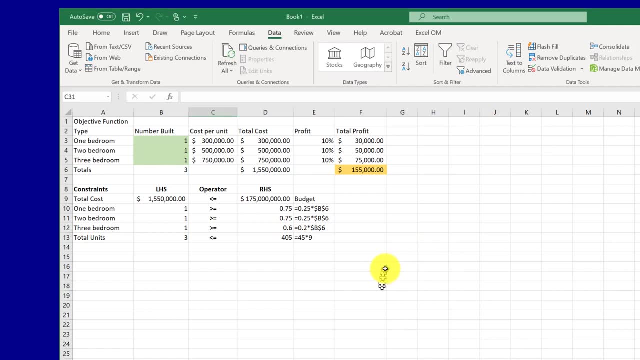 We've built the decision model and I'll walk you through how it's set up and it's designed to make it easy to plug into Solver. Okay, so here's what I've done. I built the basic model up top and I've got here the 1, 2 and 3 bedrooms, the totals, and I've set this up. 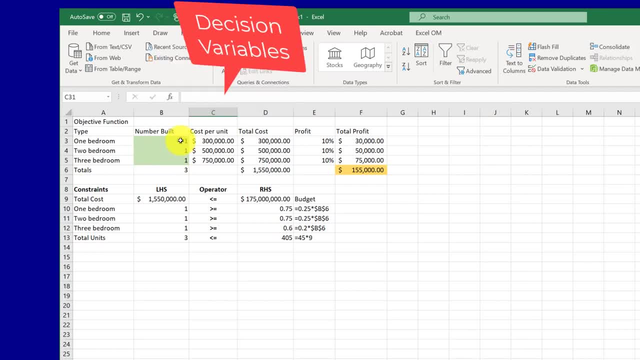 These will be the number of units that we're building, and I like to start with just putting one for those. This is the total and this is the answer of those three. You can see, that's the equation there. These are the cost per. 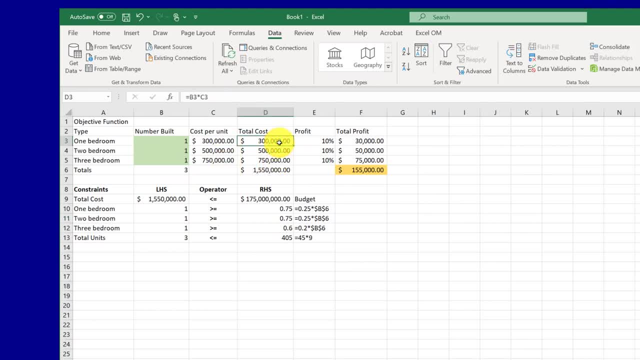 units. This total cost again has an equation there of just the number built times the cost per unit, We've got profit of 10%, and so the profit is just equal this 10% times the total cost. And we add that up to get the total profit. and here 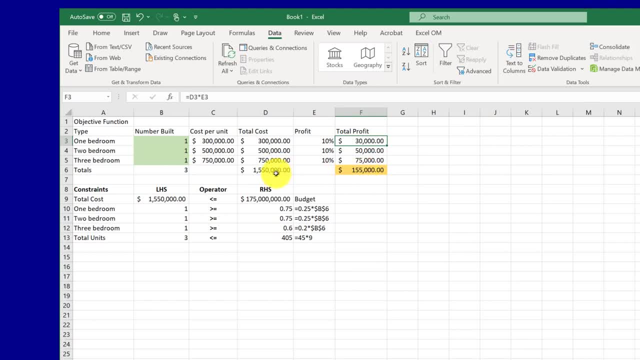 we've got our total cost. So that is our decision model and the objective function, which is this total profit that we want to maximize, built into a set of mathematical equations, Just a simple decision model. Down here I have the constraint And I like to set them up in what is known as the left-hand. 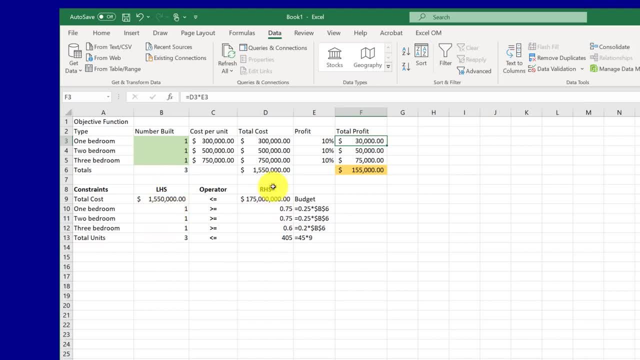 side, That's what you're constraining, And then the right-hand side has the value against which you're constraining it, And then you have a operator and then solver: It's either greater than or equal, equal or less than or equal. So I've put those in there. Total cost has got to be less than or 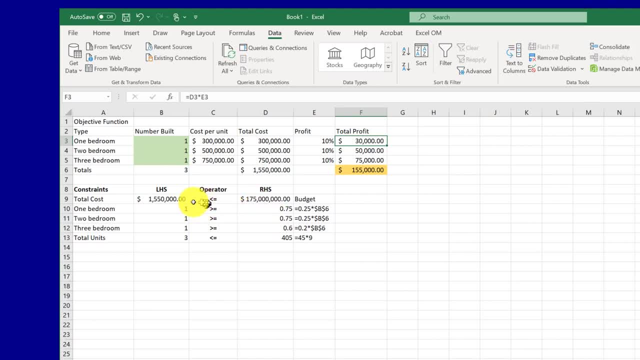 equal to the budget of 175 million dollars. And again, this cell here is just linked to that cell there to bring that down. And the same thing is true for the number of units. This is linked up to that cell And total units is linked to that cell. So I've got this decision model linked. 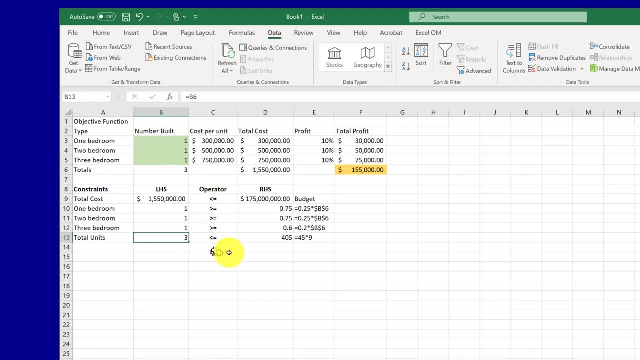 to my constraints down here. And there's again the operators And here's the right-hand side. I've got the budget. The percentage that we want to target is 25 percent of this total in B6. And again, 25 percent in the total in B6.. 20 percent. 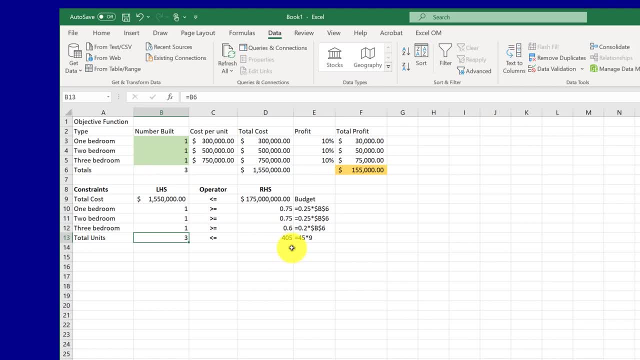 for three bedrooms minimum. And then we've got our zoning requirement. We had 45 acres with a max of 9 per acre, So 405 units is the max that we can have, And the total number of units needs to be less than or. 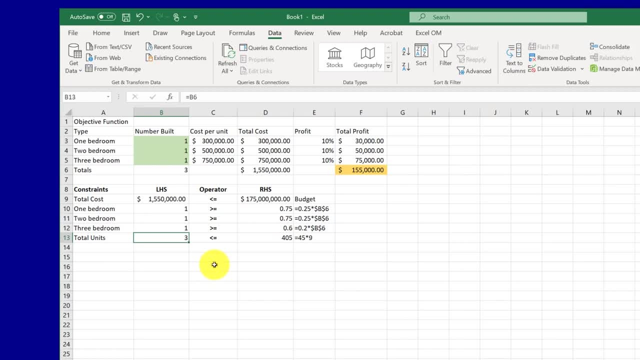 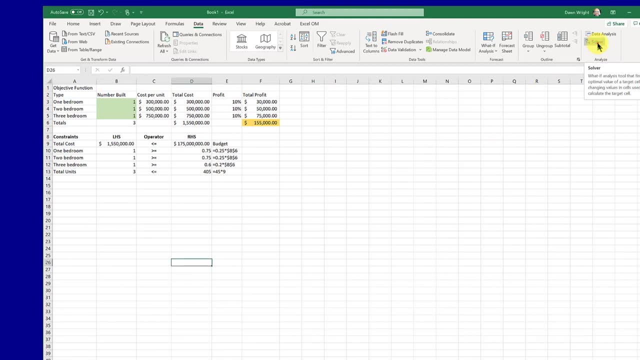 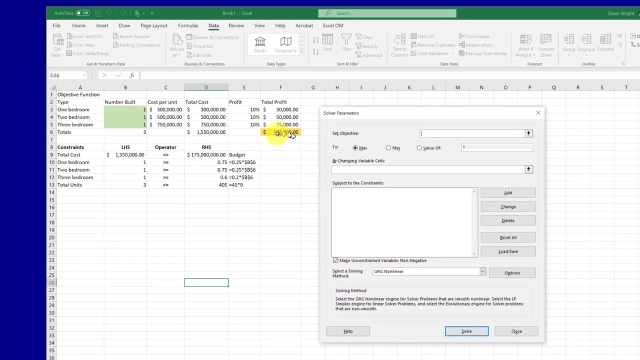 equal to that. So we've got our model and our constraints set up. Let's go to. okay, we click on solver, We get our dialog box up here, We're going to set our objective, which is 30. And then we're going to set our budget. And then we're going to set our 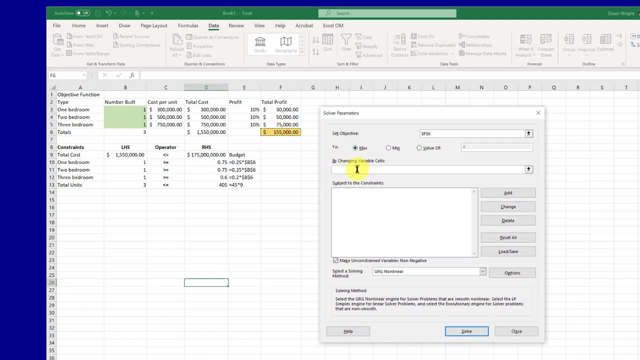 budget, That's the maximize the profit. Our decision variables: we're going to change those, That's these three cells there. And then we've got to add our constraints. So I'm going to click on add And the first constraint I'm going to add.